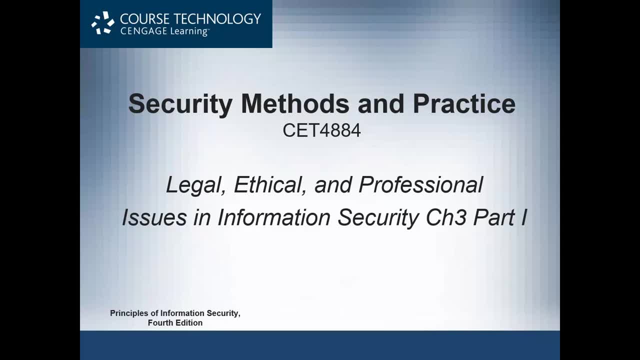 Hello and welcome to CET 4884, Security Methods and Practice. In this session we will discuss the functions of laws, regulations and professional organizations in information security and their relationship with each other. We will also address the differences between laws and ethics. 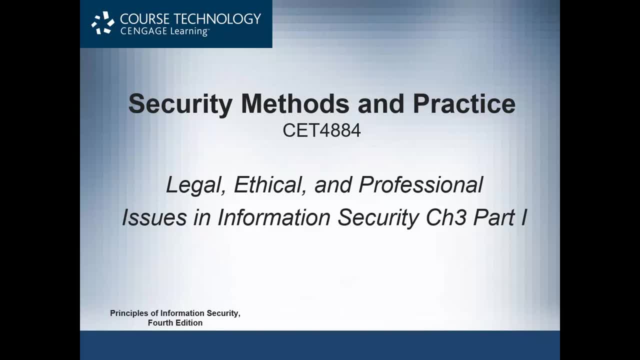 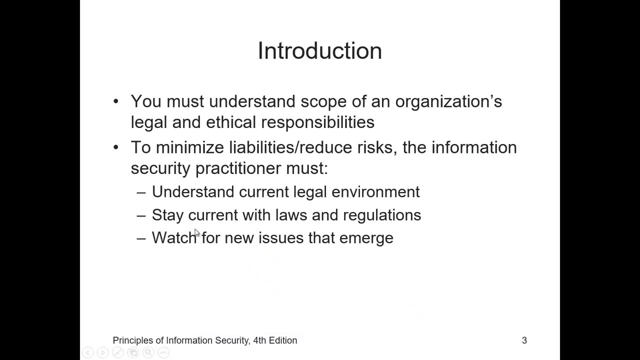 We will discuss major national laws that affect the practice of information security. In addition, this session will explain the role of culture as it applies to ethics in information security. As an information security professional, it's very important to understand the organization's legal and ethical responsibilities. 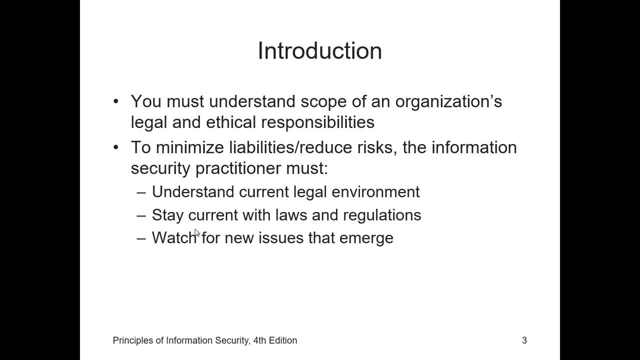 The organizational information security must be up-to-date, adhering to the latest laws and regulations. In addition, security practitioners must watch the threat issues that need attention To be vigilant and understand. the new laws will minimize liabilities, reduce risk from electronics and reduce losses from legal actions. 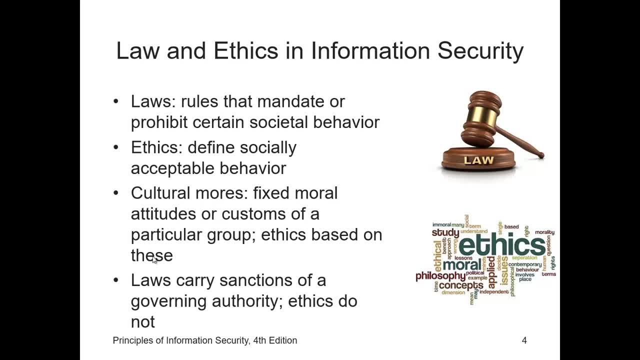 Before we go further in this chapter, let's understand the meaning of both the law and the ethics. Laws are the rules adopted for determining accepted behavior in modern society and as individuals, we elect to trade some aspects of personal freedom for social order. Laws are drawn from ethics, which are defined as socially acceptable behaviors. 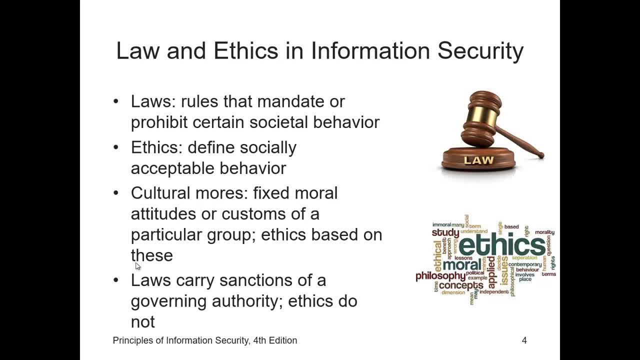 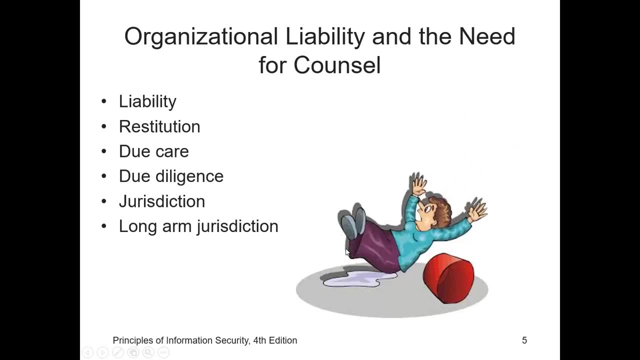 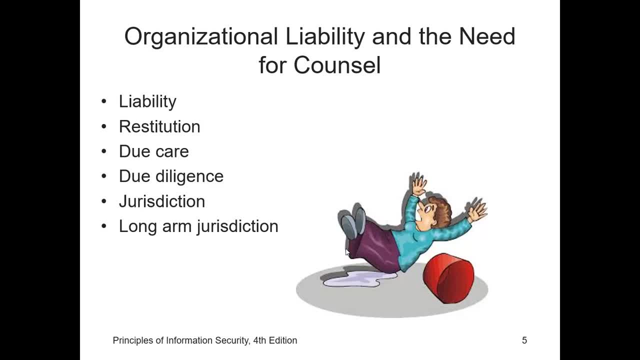 information security. the company should be liable for their customer personal information. the restitution is compensation or compensating customers for wrong committed by an organization or its employees. training should be provided to ensure that employees know what constitute acceptable behavior and know the consequences of illegal or unethical actions, ensuring that 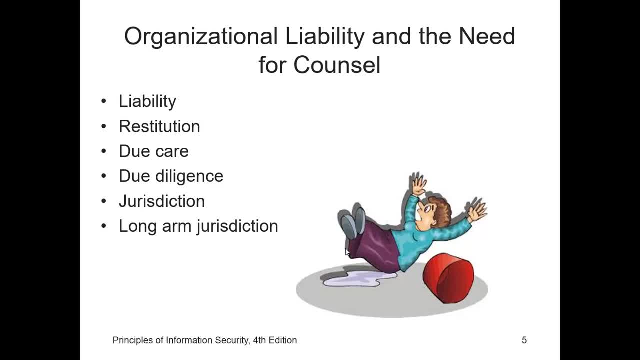 employees know what is acceptable is called do you care? while due diligence is defined as making a valid effort to ensure that the employee is doing what is acceptable and is doing what is to protect others, continually maintaining level of of effort, jurisdiction courts, right to hear a case of the wrong was committed in its territory or involved its citizen area. long arm Jesus. 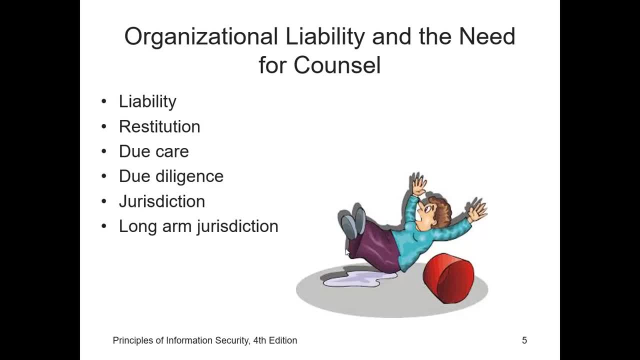 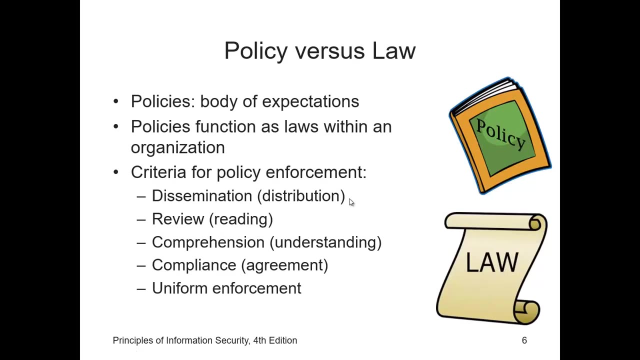 direction: right of any court to impose its authority over a individual organization if it can establish jurisdiction. we need to understand the difference, the difference between policies and laws. the policies are defined as the list of expectations that describe acceptable and unacceptable employee behavior in the workplace. policies could be considered as laws within an 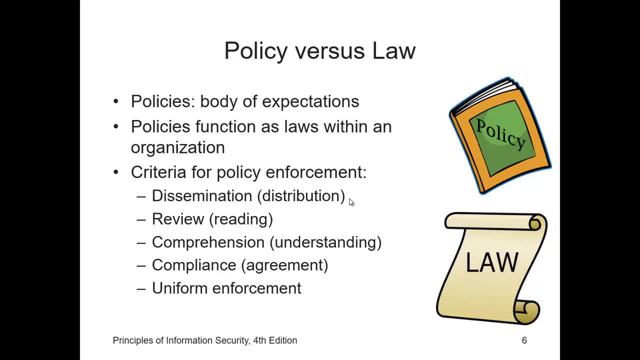 organization and must be written carefully to ensure they are complete, appropriate and fairly applied to everyone. the law is a system of rules and guidelines that are enforced on all people. to enforce policy. the written policy will be distributed to all companies employees, where they will have the chance to read it and comprehend once being read. the employees have to comply with. 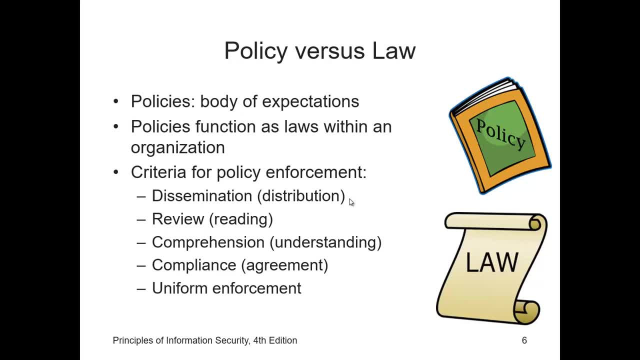 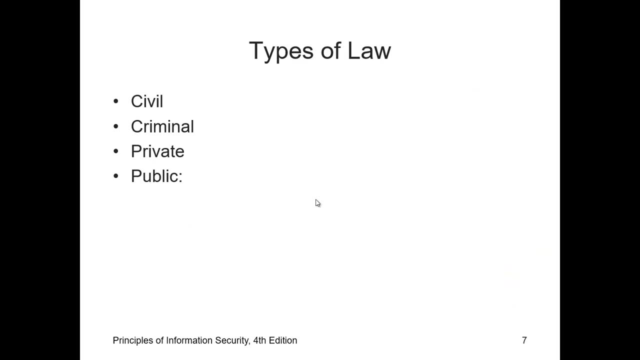 companies policy and follow this policy. once being read, the employees have to comply with companies policy and follow this policy. The enforcement will be fair, equal and uniform through all departments. There are several types of laws. We have the civil law, which represents a wide variety of laws that are recorded in volumes of legal code available for review by the average citizen. 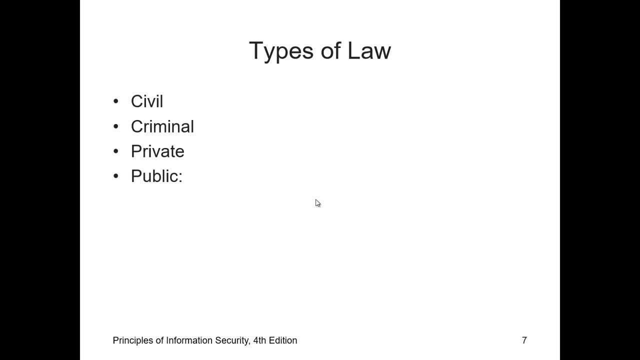 We have the criminal law, which addresses violations harmful to society and is actively enforced through persecution by the state. We have the tort law, which allows individuals to seek recourse against others in the event of personal, physical or financial injury. We have the private law. 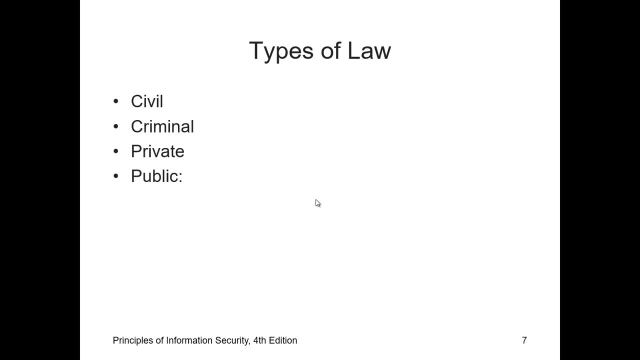 We have the private law, which regulates the relationship between the individual and the organization and encompasses family law, commercial law and labor law. The public law regulates the structure and administration of government agencies and their relationships with citizens And with, of course, the employees and the other governmental entities, providing careful checks and balances. 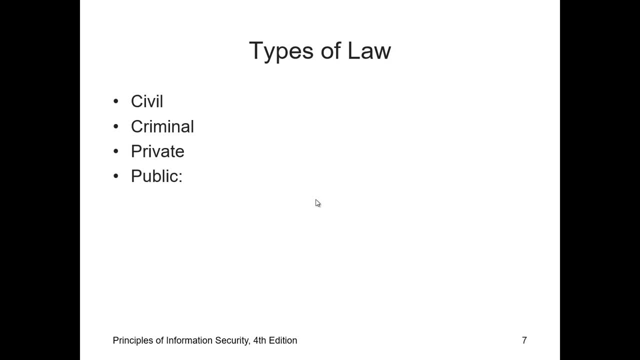 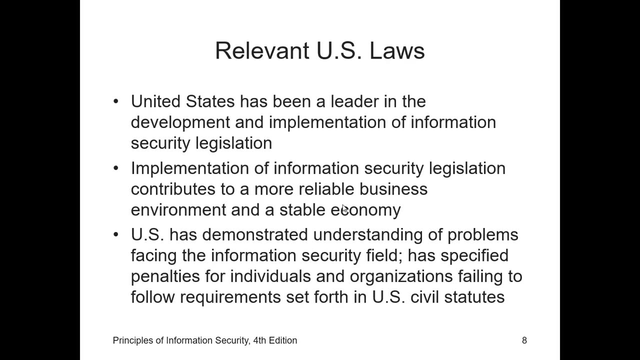 Examples of public law include criminal, administrative and constitutional law. There are lots of international laws related to information security, and the US has been a leader in the development and implementation of such laws. These laws assist in creating a reliable business environment and more stable economy. 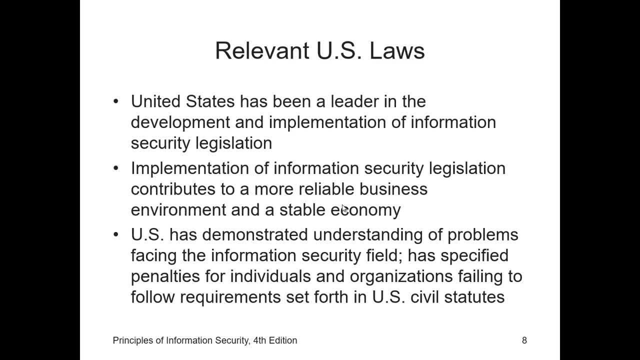 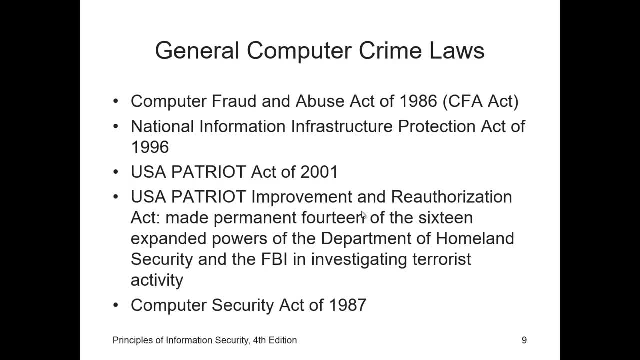 We have the public law, which regulates the administration of government agencies and their relationships with citizens. There are specific penalties for individuals and organizations failing to follow requirements set of information security laws. So what are the different US laws related to information security? 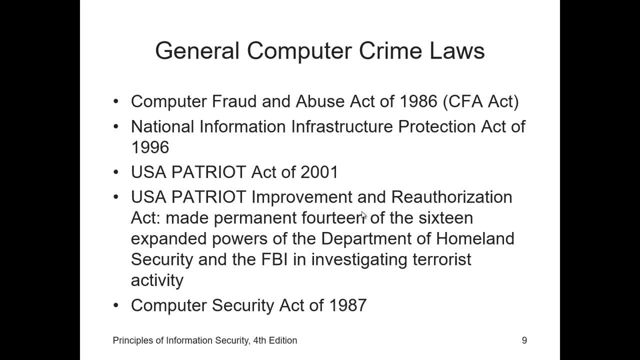 Let's start with general computer crime laws. The Computer Fraud and Abuse Act of 1986 is the cornerstone of many computer-related federal laws and enforcement efforts. It was amended in October 1996 with the National Information Infrastructure Protection Act of 1996,. 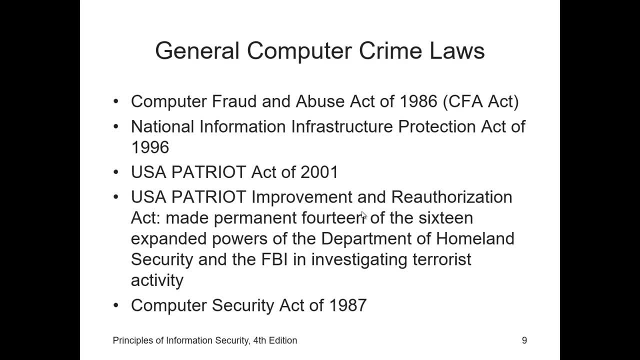 which modified several actions of computer fraud and abuse and increased the penalties for selection Evaluated crimes, severity of penalties judged on the purpose of commercial advantage, private financial gain and in furtherness of a criminal act. The USA Patriot Act of 2001 modified a wide range of existing laws to provide law enforcement agencies. 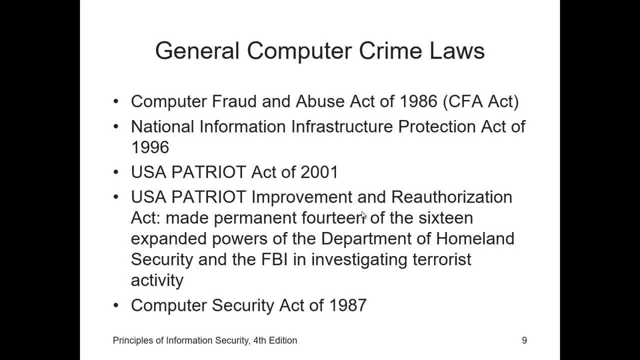 with a broader latitude of actions to fight terrorism related activities. The Communication Act of 1934 was revised by the Telecommunication Deregulation and Competition Act of 1996, which attempts to modernize the archaic terminology of the older Act. These much-needed updates of the terminology were included as part 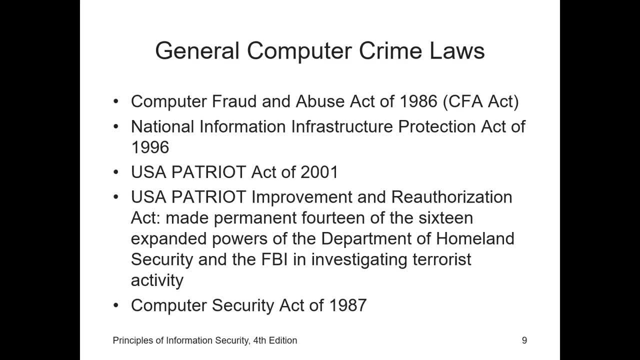 of the Communication Decency Act. The CDA was immediately trapped in a spiky legal debate over the attempt to define indecency and ultimately rejected by the Supreme Court. Another key law that is of critical importance for the information security profession is the Computer Security Act of 1987. It was one of the first attempts. 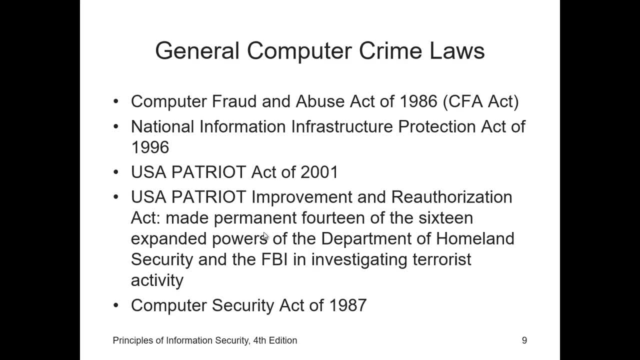 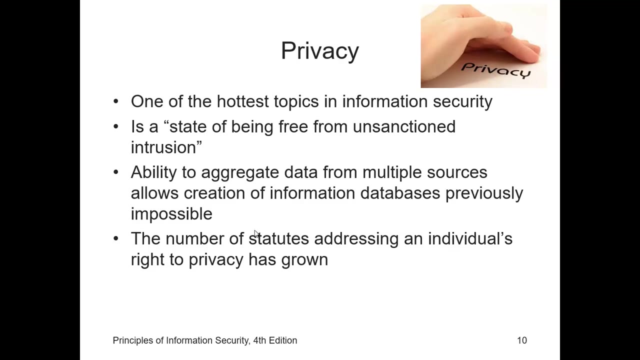 to protect federal computer systems by establishing minimum acceptable security practices. The National Bureau of Standards, in cooperation with the National Security Agency, became responsible for developing these security standards. Information privacy is an important issue and has been discussed widely recently. The ability to collect information on an individual, combine facts from separate sources or resources. 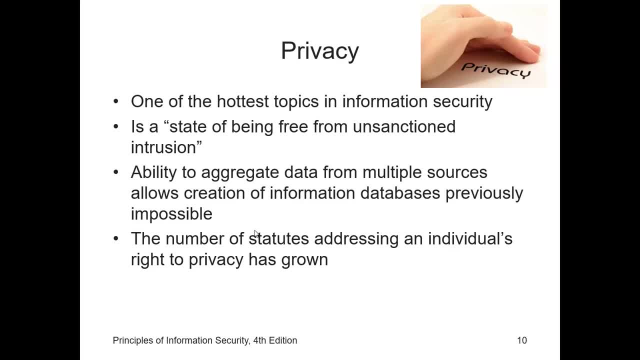 and merge it with other information has resulted in databases of information that were previously impossible to set up. The aggregation of data from multiple sources permits unethical organizations to build databases of facts with frightening capabilities, And you can watch the video provided about privacy to see you know: it's not you know. 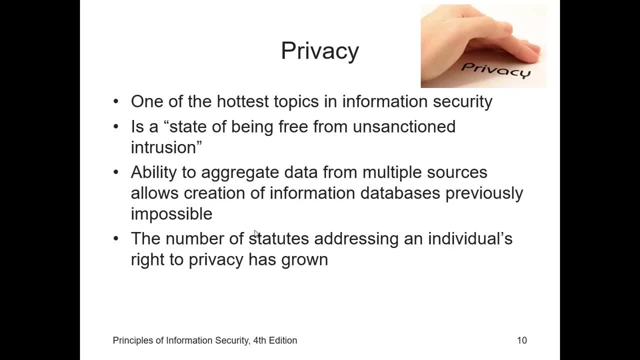 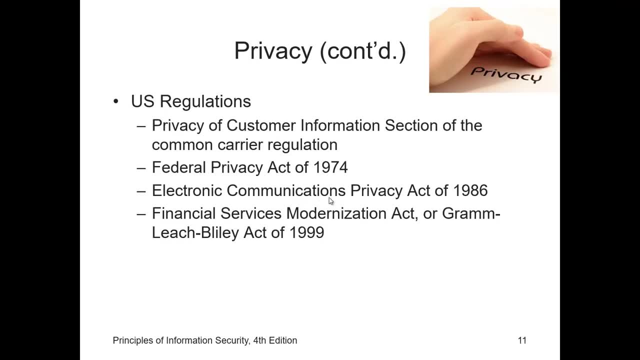 real. but you know, imagine if that would happen. It's it would be so scary to think like that. The buyer pays. the Hannock Report givesiro concession says it is intangible and he says there are three options: an income insurance had rewards from office hours which he might. 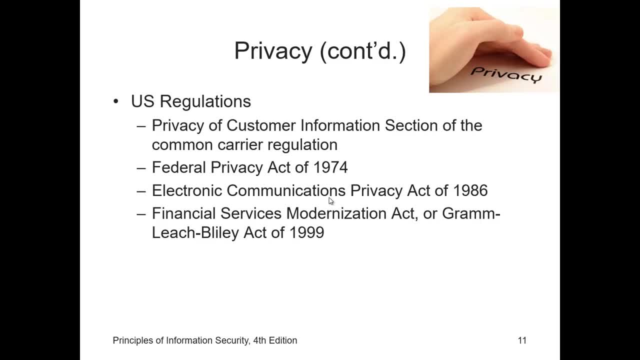 be. think, because there are security options, an excuse and a warranty, Slap it around the neck? yes, it does- would make a great deal of sense for the immigration company. certainly There are a few greatINAW signed府S regulations that ensure individual privacy. One of the 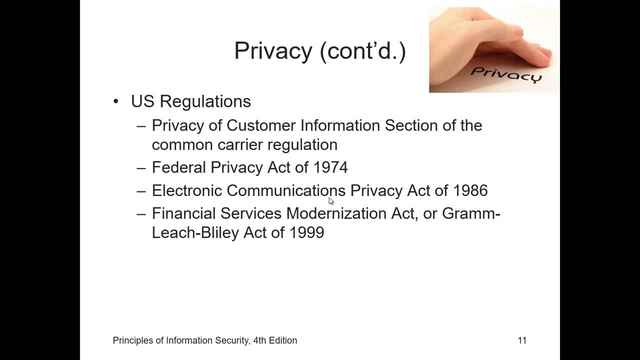 most common rules is that privacy of customer information section of common career regulation- cannot disclose this information except when necessary to provide their services. The only other exception is when a customer requests the disclosure of information and then the disclosure is restricted to that customer's information only. 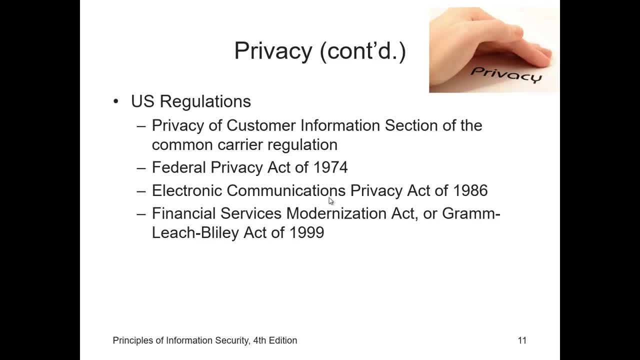 The Federal Privacy Act of 1974 regulates the government in the protection of individual privacy and was created to ensure that government agencies protect the privacy of individuals and businesses information and to hold those agencies responsible if any portion of this information is released without permission. The Electronic Communication Privacy Act of 1986 regulates the interception of wire. 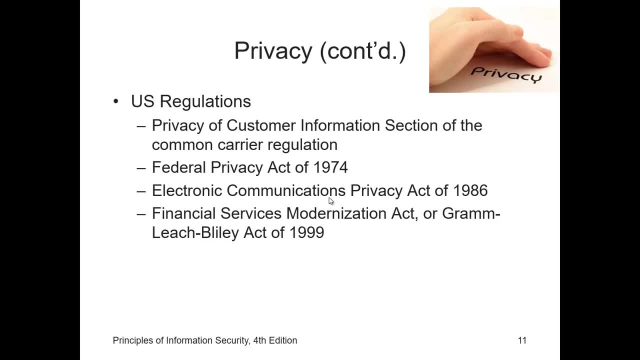 electronic and oral communications. The act works in conjunction or conjunction with the Fourth Amendment of the United States Constitution, which provides protections from unlawful search and capture. The Financial Services Modernization Act, or Graham-Leach-Billy Act that was in 1999, requires all financial institutions to disclose their privacy policies. 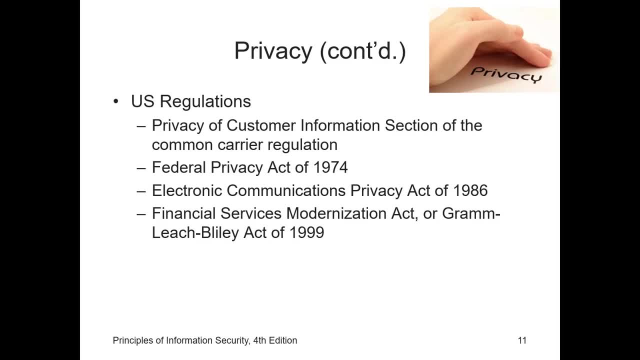 and a way of sharing those non-public personal information with the users. It also requires due notice to customers so that they can request that their information not be shared with third parties, And that's why, in most cases, you receive those information from your bank, from your credit. 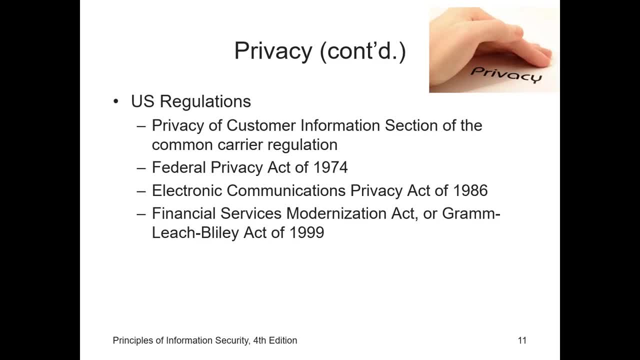 card, from even the Internet provider or from your bank. The Federal Privacy Act of 1986 regulates the interception of information and to hold those agencies responsible if any portion of this information is released without permission. The Financial Services Modernization Act of 1986 regulates the interception of wire electronic. 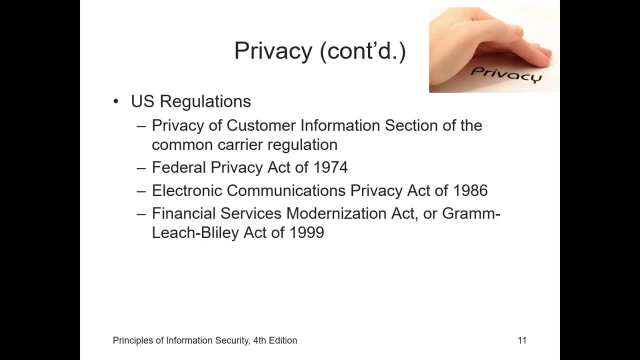 and oral communications. It also requires due notice to customers so that they can request that their information not be shared with third parties, And that's why, in most cases, you receive those information from your bank, from your credit card, from even the Internet provider or the wireless phone provider. 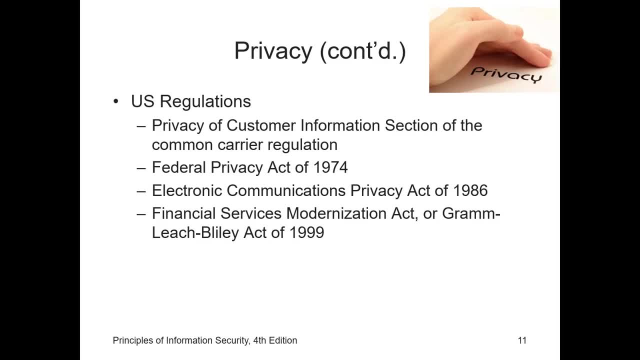 They have to provide you with this information and they have to make sure that you agree or disagree on sharing the third-party information, your information- with a third-party company. So the act ensures that the privacy policies in effect in an organization are fully disclosed when a customer initiates a business. 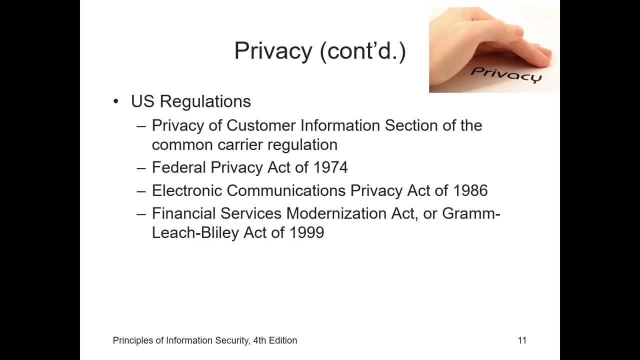 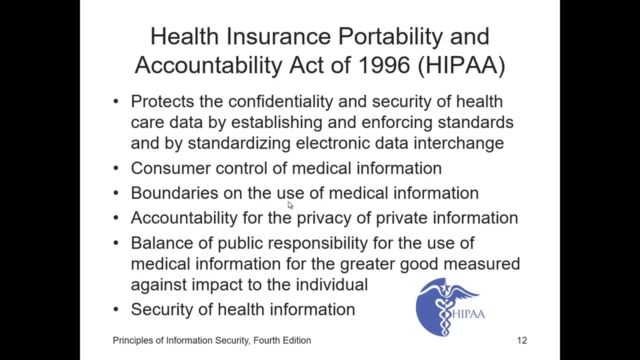 It's also recognized under the US law that when a customer begins a business, it requires the professional's permission to send its information to the individual that is in the organization. The Federal Privacy Act of 1986 regulates the interception of information from your. 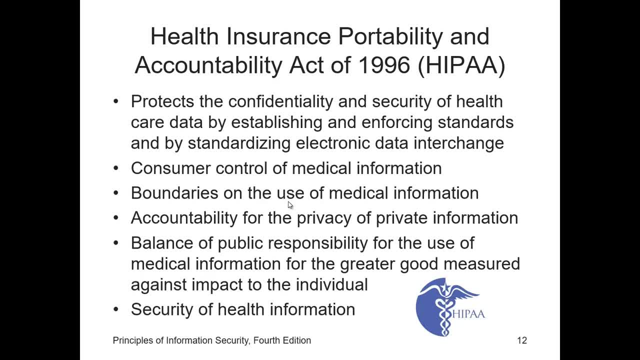 bank from your credit card. from your credit card, from your personal data, from your bank account Act. This Act impacts all health care organizations, including small doctor practices, health clinics, life insurance and universities, as well as some organizations which have self-insured employee. 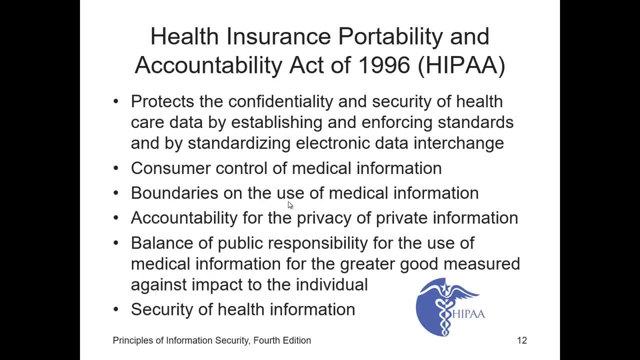 health programs. The Act requires organizations that retain health care information to use information security mechanisms to protect this information, as well as policies and procedures to maintain this security. It also requires a comprehensive assessment of the organization's information security systems, policies and procedures. There is no specification of practical 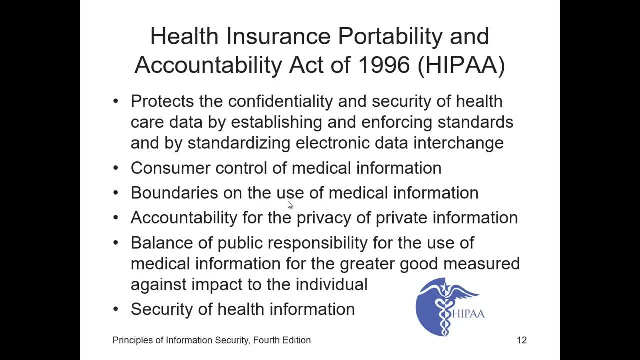 or particular security technologies for each of the security requirements, only that security must be implemented in the context of an organization. The Act also requires organizations to maintain implemented to ensure the privacy of the health care information. The privacy standards of HIPAA severely restrict the dissemination and distribution of private health information. 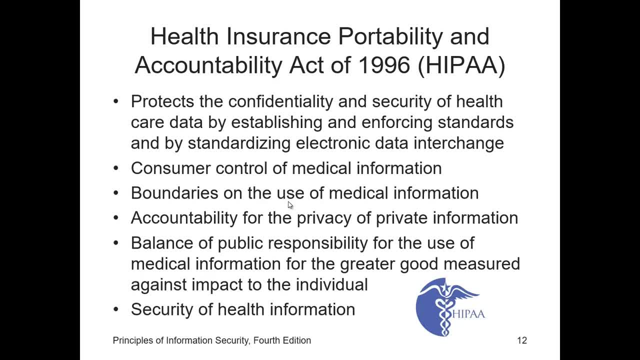 without document consent. The standards provide patients the right to know who has access to their information and who has accessed it, and also restrict the use of health information to the minimum required for the health care services requirements only. And again, if you work in a hospital as a security officer, you will sign a HIPAA. 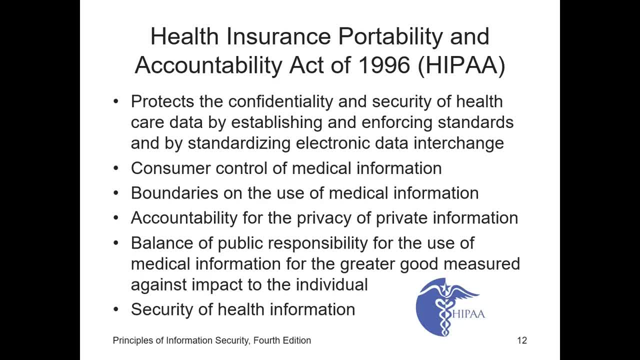 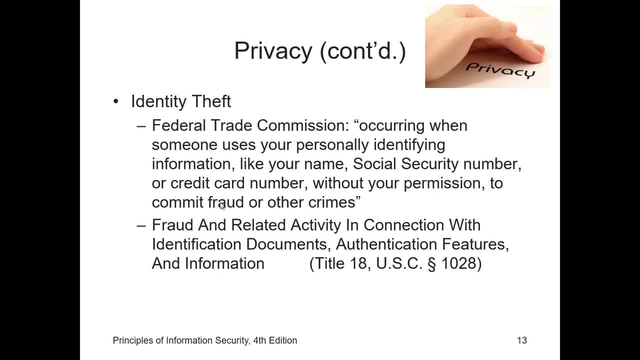 agreement not to release any information that you see or database that you see for patients. The access to customer personal information could lead to identity theft, which occurs when someone uses your personal information, such as your name, social security number and credit card number, without your permission to commit fraud or other crimes. 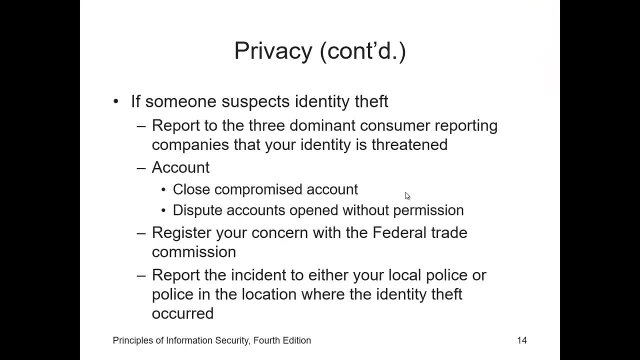 If you suspected identity theft, you have to report to the three dominant consumer reporting companies- Equifax, Experian and TransUnion- that your identity might be stolen, Close compromised accounts and dispute any new accounts that have been opened without your permission. 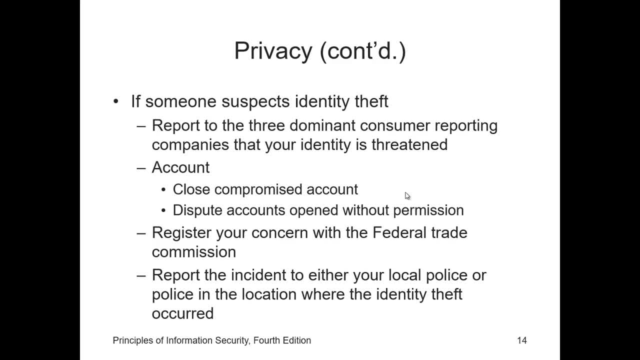 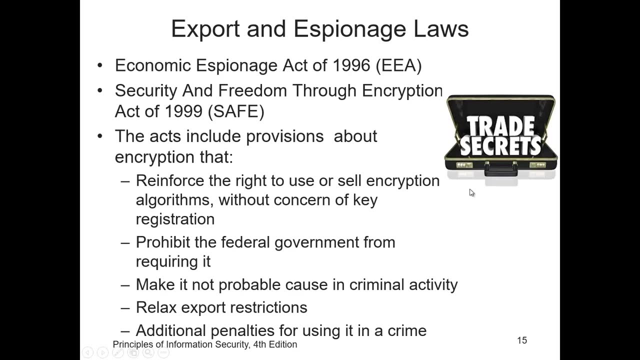 Register your concern with the Federal Trade Commission And report the incidents to either the local police or the police in the location where the identity theft happened. On the other hand, there are export and espionage laws to protect businesses In an attempt to protect American ingenuity. intellectual property- and competitive advantage. the Federal Trade Commission has issued a law that requires azul- الذي appears to be in the national минимum of steam, which is to prevent trade secrets from being illegally shared- The Economic espionage law provided by the Federal Trade. 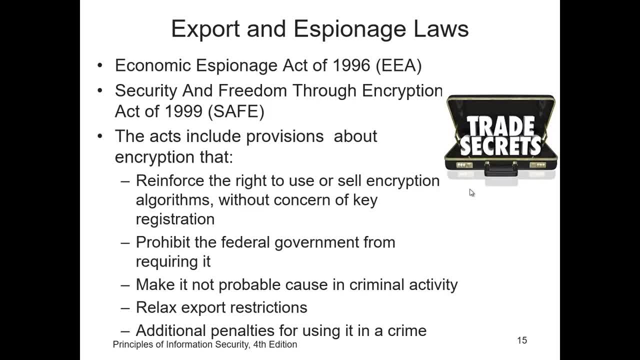 Commission and the Federal Trade Commission was introduced in 1996.. Your information is more than enough. The last act in which Congress passed the Economic Espionage Act in 1996.. This law attempts to prevent trade secrets from being illegally shared. The Security and Freedom through Encryption Act of 1997 was an attempt by Congress to 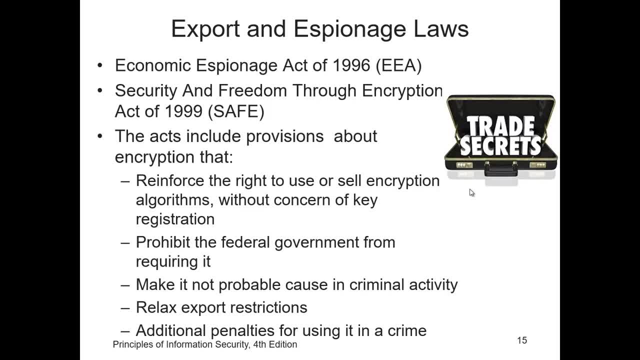 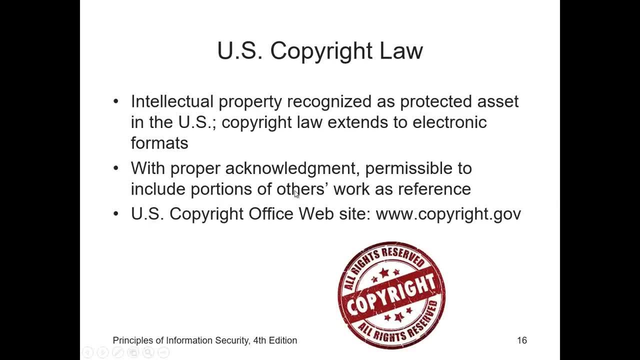 provide guidance on the use of encryption and provided measures of public protection from government intervention. The act is successful intervention US copyright law and we all for sure heard that and we know it. it's, as stated in a previous lecture, business intellectual property that has been targeted by hackers and, as a result, intellectual property is recognized as protected assets in the US. 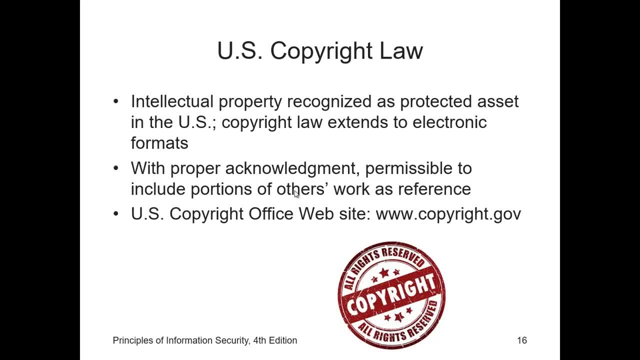 So, basically, the US copyright law extends this right to the published word, including electronic formats. The fair use of copyrighted materials includes the use of the, the use to support news, reporting, teaching, scholarship and a number of other related permissions, so long as the purpose of the US 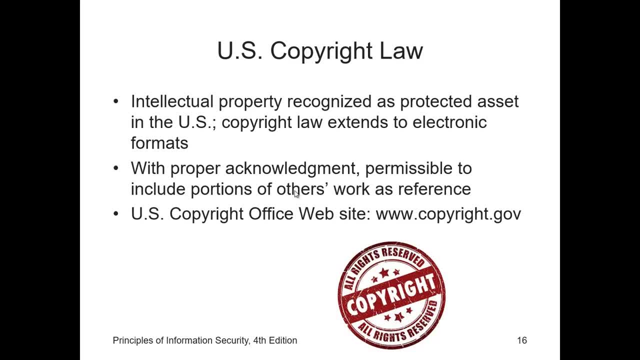 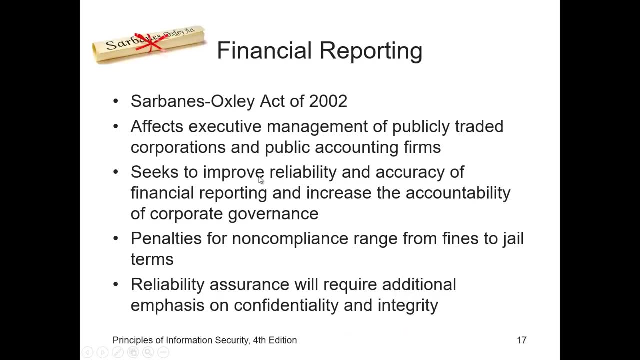 use is for educational or library purposes, not for profit or any other excessive use. From the financial side, there was the Sir Baines-Oxley Act of 2002, which included reforms in corporate governance and the accounting profession. The reform or the act intended to improve corporate financial reporting and internal control, strengthen audit committees, change the relationship between the auditor and client, improve auditor independence, provide additional auditor assurance of our internal control, provide oversight and regulation for auditors or publicly traded auditors. 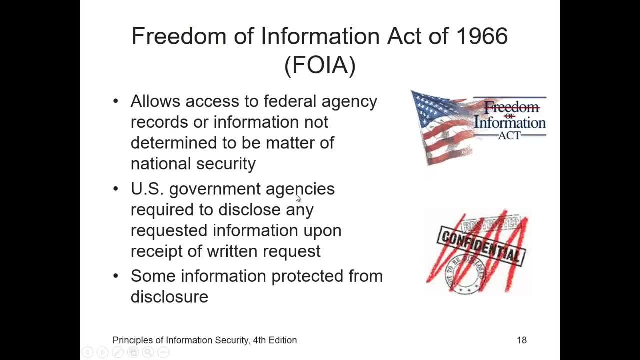 companies. The Freedom of Information Act of 1966 provides any person with the right to request access to federal agency records or information not determined to be a matter of national security. US government agencies are required to disclose any requested information. on receipt of written. 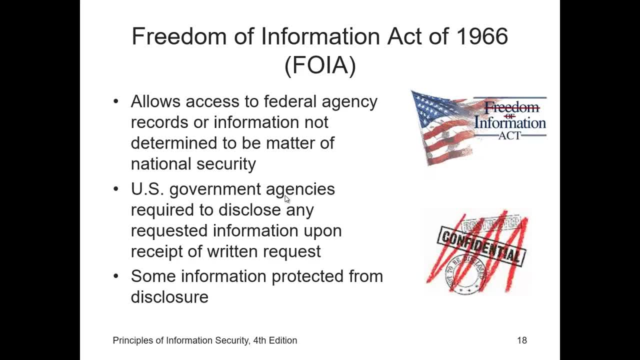 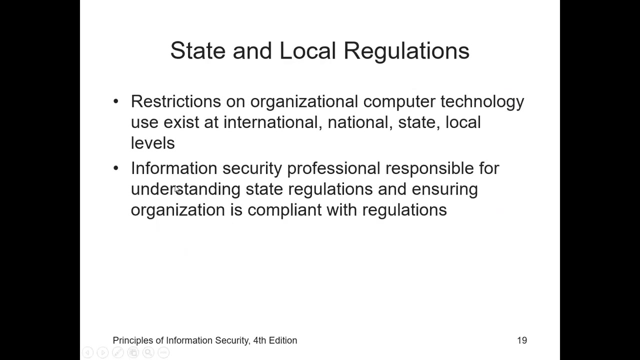 request. There are exceptions for information that is protected from disclosure, and the Act does not apply to state or local government agencies or to private businesses or individuals, although many states have their own version of the Act, In addition to the national and international restrictions placed on an organization. 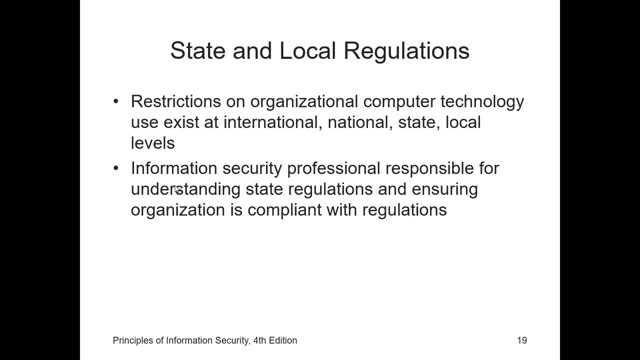 in the use of computer technology. each state or local entities, local agency may have a number of laws and regulations that impact operations. It's the responsibility of the information security professional to understand state laws and regulations and ensure the organization's security policies and procedures comply with those laws and regulations. 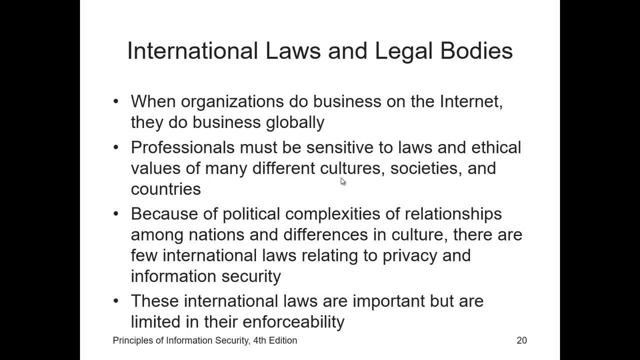 Companies outsource their operations and produce their product overseas. In addition, they sell their products using Internet. Companies are not limited to a certain location within one country. They are globally connected to the international community. So in this case, we need to extend the laws to. 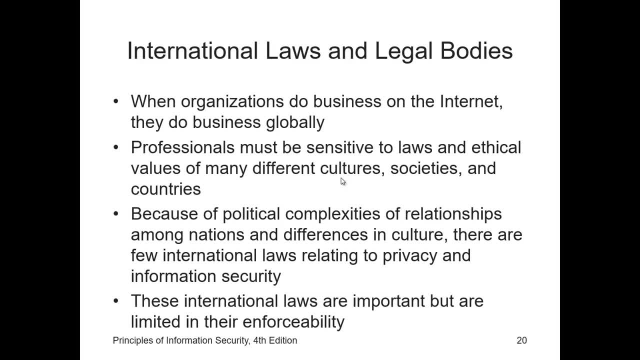 the international laws and make sure that we cover the company's policies and procedures also as international laws. So, based on that, professionals must be sensitive to laws and regulations and regulations. In addition, we must protect businesses from both sides. In addition, due to the political complexities and 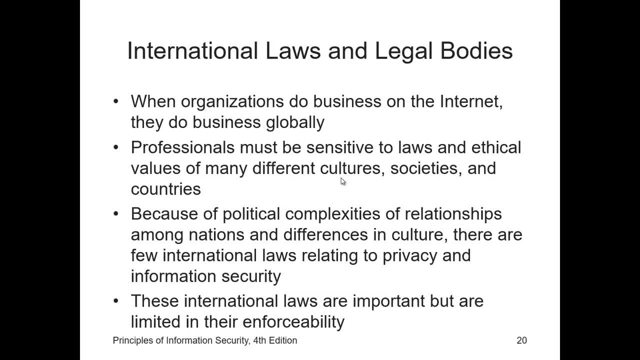 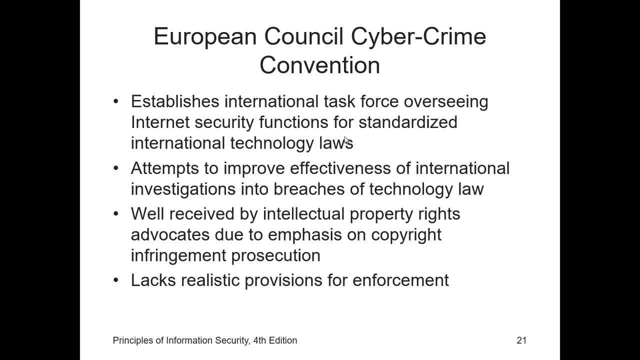 cultural differences, there should be international laws to protect businesses from both sides. Although these international laws are important, they are limited in their enforceability, unfortunately. Recently, the Council of Europe and the Council of Europe drafted the European Council Cybercrime Convention, designed to create an international task force. 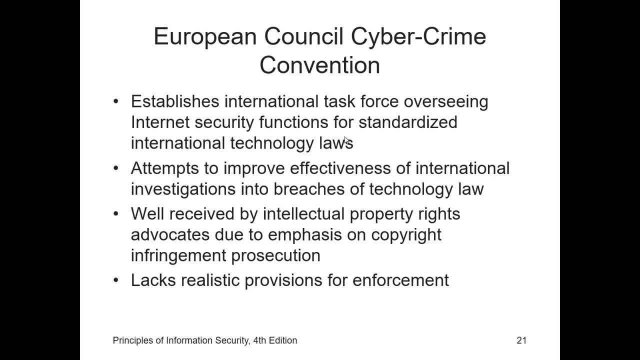 to oversee a range of security functions associated with Internet activities and to standardize technology laws across international borders. It also attempts to improve the effectiveness of international investigations into breaches of technology law. This convention is well received by advocates of intellectual property rights, with its emphasis. 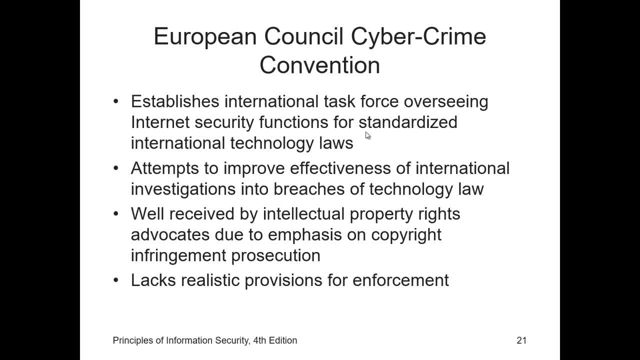 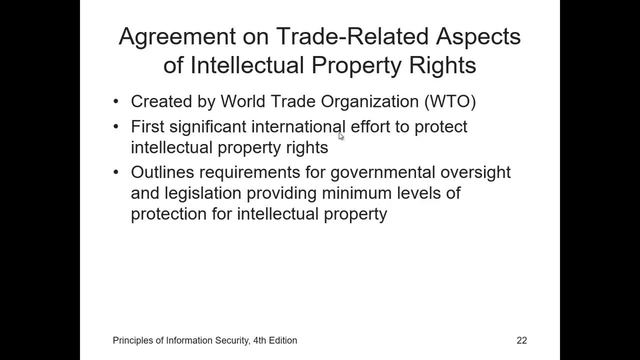 on copyright infringement prosecution. Another international collaboration is the Agreement on Trade Related Aspects of Intellectual Property Rights that was created by the World Trade Organization. The agreement drafted the first significant international effort to protect intellectual property rights. It outlines the requirements for governmental oversight and legislation providing minimum 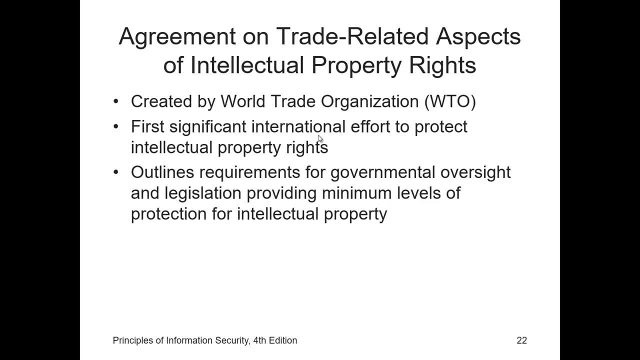 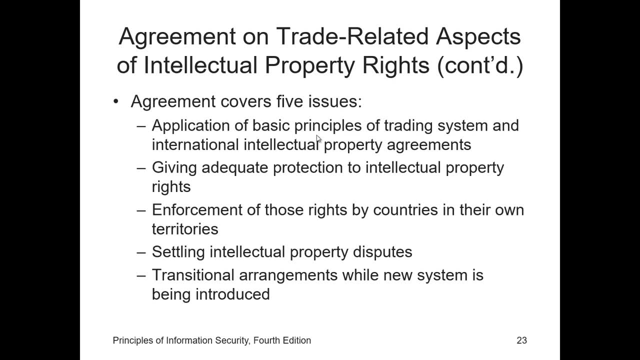 levels of protection for intellectual property Agreements covers five issues: Application of basic principles of trading system and international intellectual property agreements. giving adequate protection to intellectual property rights. enforcement of those rights by countries in their own territories. settling intellectual property disputes. and 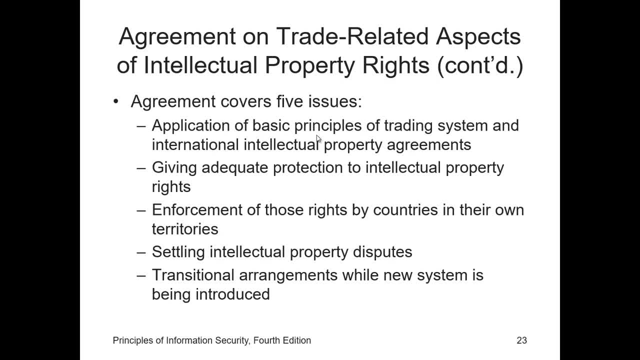 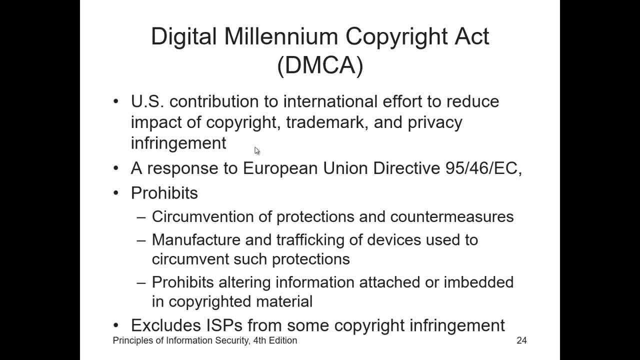 transitional agreements while new system is being introduced. The Digital Millennium Copyright Act is the United States version of an international effort to reduce the impact of copyright, trademarks and privacy infringement, especially through the removal of technological copyright protection measures. The European Union also put forward Directive 9546 EC.